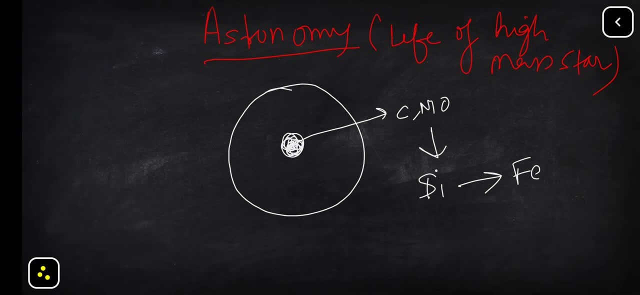 hi everyone. so in this video we will discuss about life of a high master, how the life of a high master goes on. so we discussed that in low master the central core will form the carbon nitrogen oxygen and with that the life of the low master ends. but it does that so in very longer time, say 10 billion years. okay, 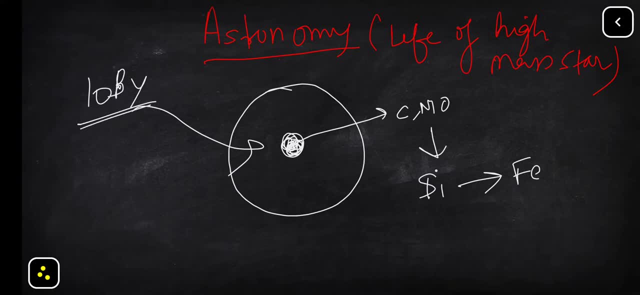 but high master will reach to this stage in very less, like hundred million year only. okay, so when the high master will raise to this, reach to this end of the cycle, then what happens? this high masters, because they have low, more matter inside them, right? so that's why this core will be even bigger. so this bigger core and 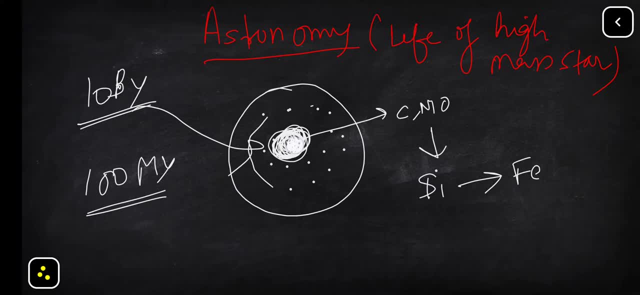 heavier code with lead to more contraction. it will lead to more contraction, right, it will lead to more contraction of this core inside and, due to this, temperature will increase. and temperature increase means because this gas is needed in this, elements need more temperature to change to higher elements, to silicon or, and then silicon to iron. so 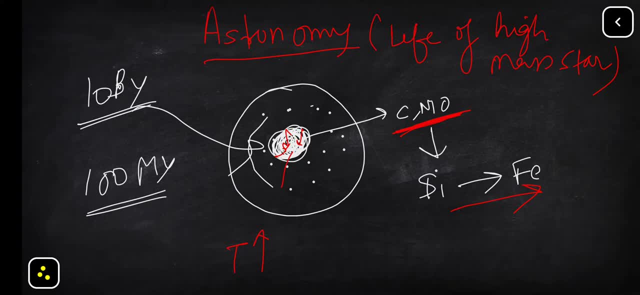 at that point- star is still not dead till later now- and it start to fuse helium- sorry, iron, silicon and iron. but then what happens is that when this iron is formed, iron can no longer do any more, can form any heavier element right under the only the influence of temperature or more gravity. 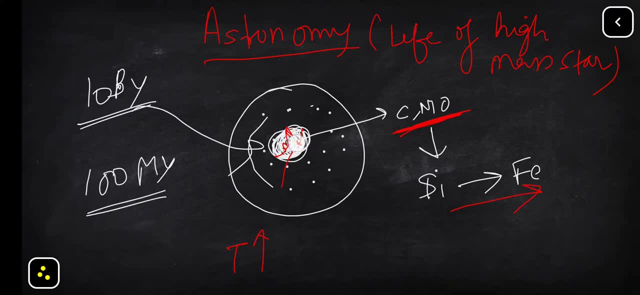 salt. so what happens? the whole will keep on collapsing, collapsing, collapsing. wait till a point where all the electrons will combined with the proton to make one, make on the troki's all the matter, all the because this central thing is sodimensional- a Era, and then certainly bust, burst out because there is a 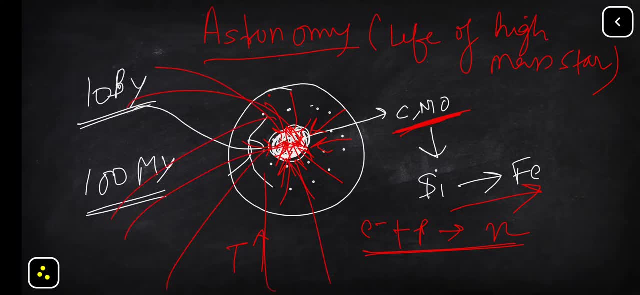 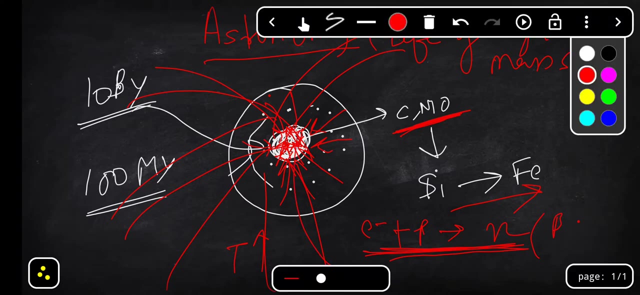 a, because there is no more contraction that can happen at neutron stage. right, because neutron is a baryon and baryon degeneracy pressure will stop it from further collapsing. so when this thing happens, right, this is called a supernova. so all the collapsing part of the star suddenly falls towards the core, even the 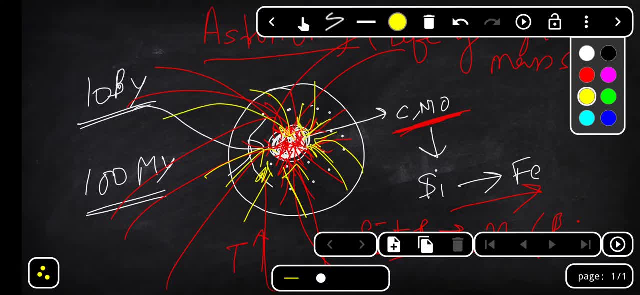 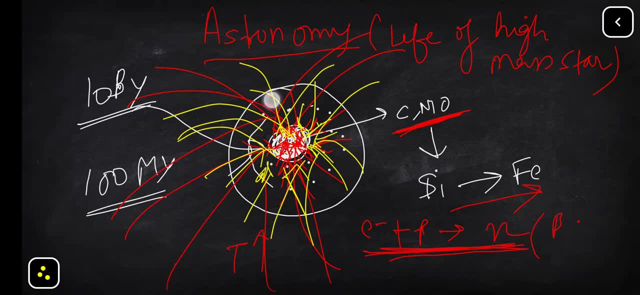 core itself and it bounces off. it bounces off suddenly, okay, it bounces off suddenly from this core in a gigantic explosion called supernova. this thing is called supernova and it is specifically called type 2 supernova. so because all the things are suddenly bursting out, 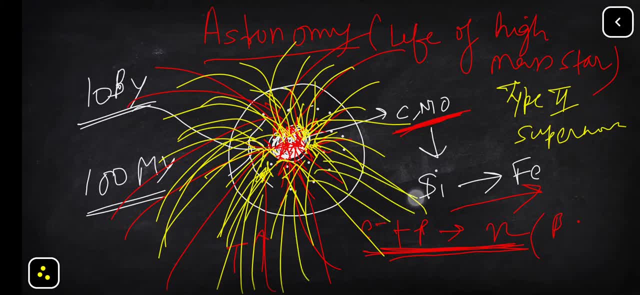 with a lot of energy. it is very luminous and very energetic, so this marks the death of a high-mass star. they literally die in a type 2 supernova. okay, supernova is just a wave which matters in, fall and then suddenly burst out with. 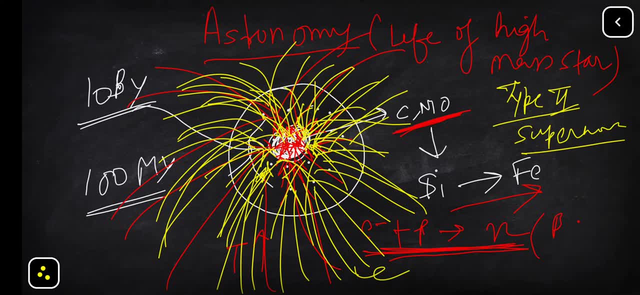 the higher energy because of this pressure of neutron will not allow them to further collapse at some point. with a given mass, it will not allow, right? so this is type 2 supernova. they are type 1 supernova also, but we will discuss it later. and more serious case of this is when the mass of star is so much that 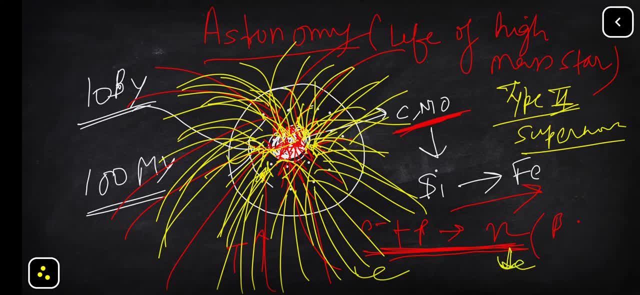 this neutron degeneracy can also not stop the collapse, and then it forms what you know as black hole. so all the matter will collapse in one single pinpoint area, right, and that is called black hole, black hole. but this is how black holes are formed, okay, and this is. 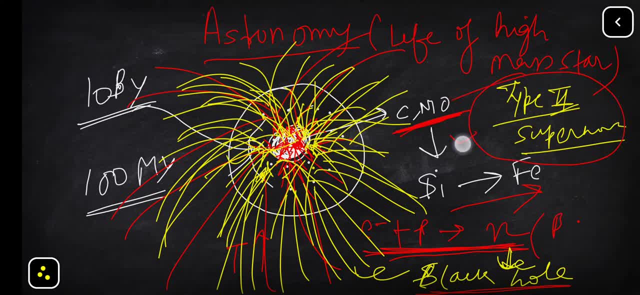 how supernova occurs. okay, so supernova will leave the central core, which is of all neutrons, that is, that is called a neutron stars. okay so. type 2 supernova, black hole and neutron stars are all formed from collapsing stars. I think you know this now better. now, what is type 1a supernova? okay, so. 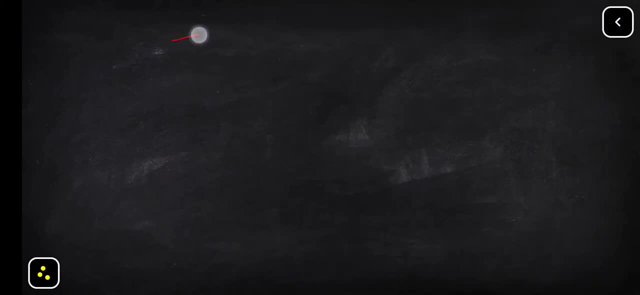 type 1a supernova. type 1a supernova is when there is a white dwarf. I told you. the white dwarf is simply the low mass star which has only carbon nitrogen oxygen left in its core. okay, and because it is not so massive, it is not able to further fuse any other. 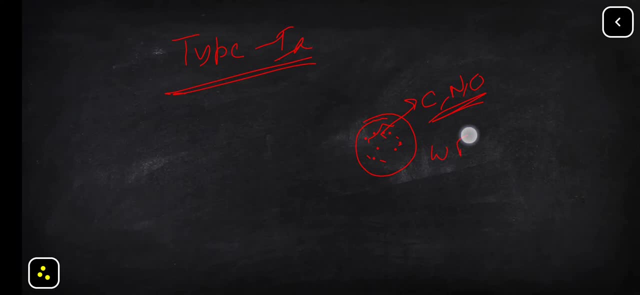 elements. but if this white dwarf- this is white dwarf- and suppose there is a star nearby which is a dielectric gas, dielectric star of very high mass, okay, suppose these are in binary. so what happens if they are near apart? this white dwarf will accrete matter from this star. okay, and when? this 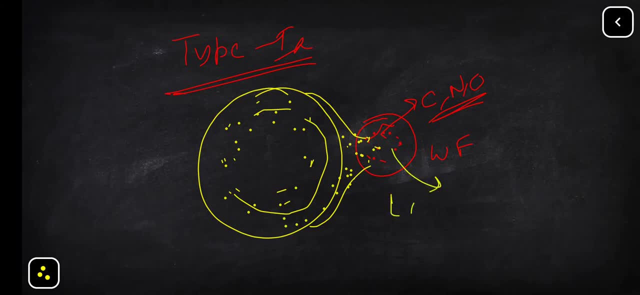 limit. when this mass of the star limit- this is a limit of 1.44 times mass of the Sun, or more than that. this is called Chandrasekhar limit- then this star also explode. right, this star also explode because now it will again collapse to, will start collapsing and this collapse will lead to same reaction that was happening. 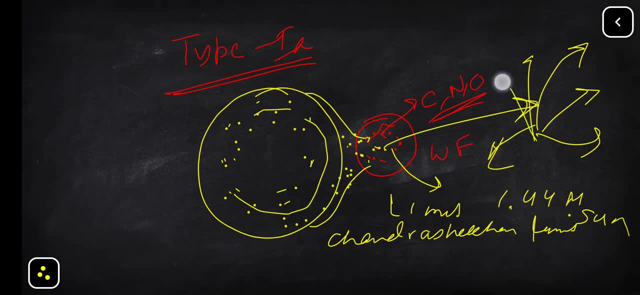 in high mass stars, but this will again collapse and then collapse and with the further collapse it will bounce back as a high energy, as when high energy will be released because that is certain collapse from a central neutron region or some other region. okay, this is type 1a supernova, that was type 2 supernova, so type 1a supernova will. 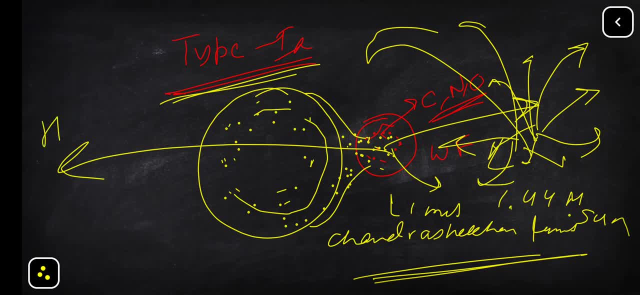 not have any hydrogen in it, because we knew that type 1a supernova is formed when carbon hydrogen oxygen central core is accreting more hydrogen or more element from here. so this will not will have more, not will have the hydrogen in its main content. 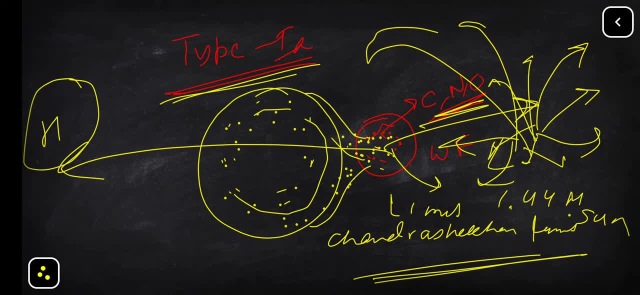 while type 1- 2a supernova will have more amount of hydrogen in its outside concentric ring and that will will be seen in this spectrum. so that's why how we demarcated from type 1a supernova and type 2 supernova. 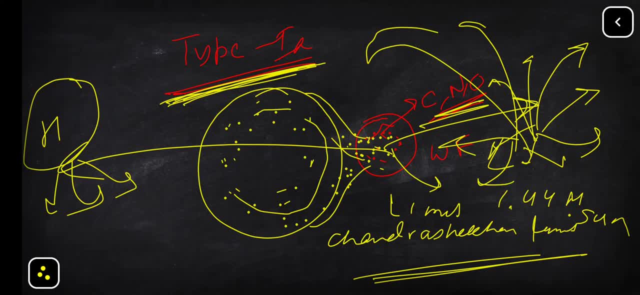 okay, so i think you know now about the type of supernova. and one more thing is: this type of supernova is known as standard candle. standard candle because they emit energy with a fixed amount of luminosity, so which with which we can know how far they are actually. i'll talk. 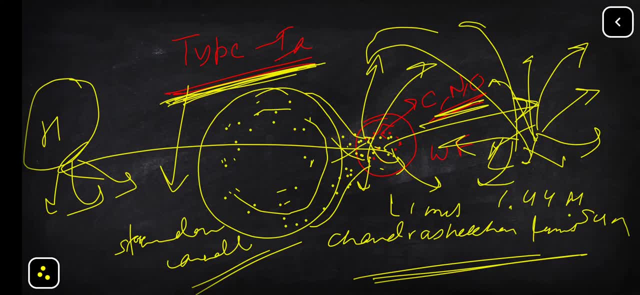 about that later in the next video. so that's how supernova is formed, and this is type 2. the supernovas are formed, the black holes and neutron stars are formed. okay, so one more thing is: this supernova can be used to detect the ancient star. 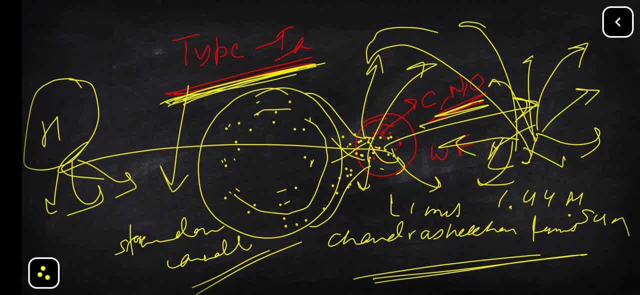 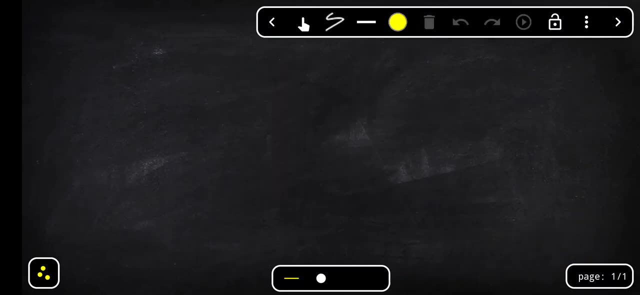 formations and because the core, the leaf, like, if you find, find somewhere the neutron star, you can say that at this place supernova might have happened right and it will also have a. it will also have some. it will also have some area which is like the gas cloud is, or the energy from the central supernova is. 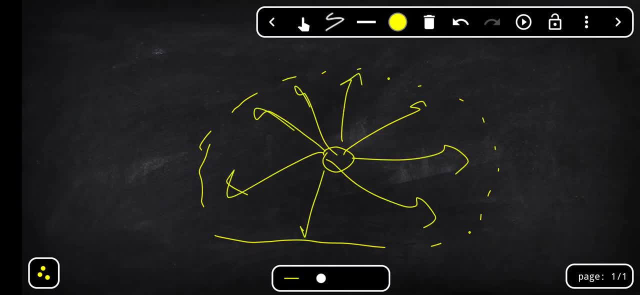 like going away. so because in space this will be someday the 10 light-year, 100 light-year, 1000 light-year, something, so we can know from that that how much light years ago, how much years ago central star has collapsed, because we will see a ring.